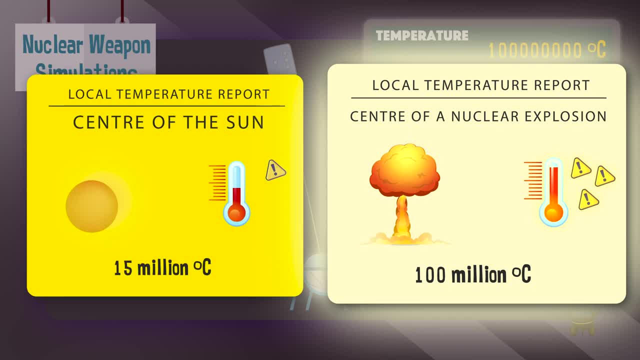 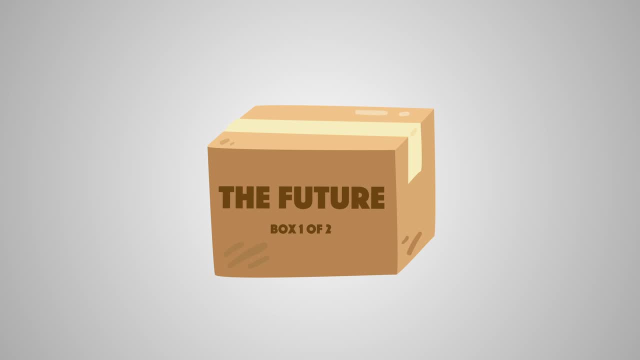 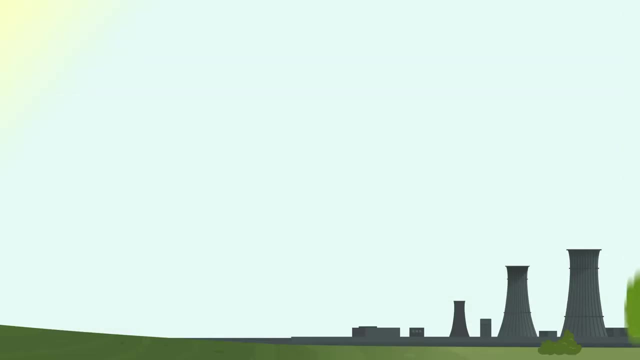 Now that's far hotter than the centre of the sun, And this type of research is also being used to better technology, helping mankind move into the future. But how exactly? How would this help anyone? Well, through something called fusion, But we'll get into that a little later. For now, let's talk about fission and how it produces. 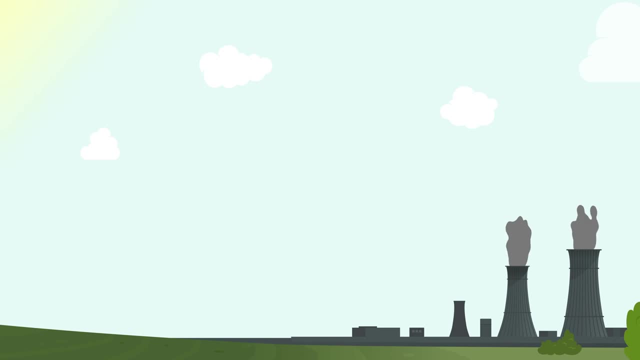 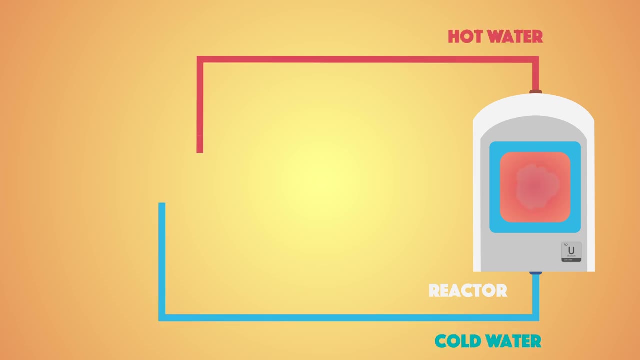 energy for nuclear power. So how does it work? By splitting uranium atoms, you can produce a tremendous amount of heat. Now, when this is contained correctly, you can circulate water around it, which, of course, turns to steam with enough heat. Now, with this steam, you channel it through a turbine and voila. 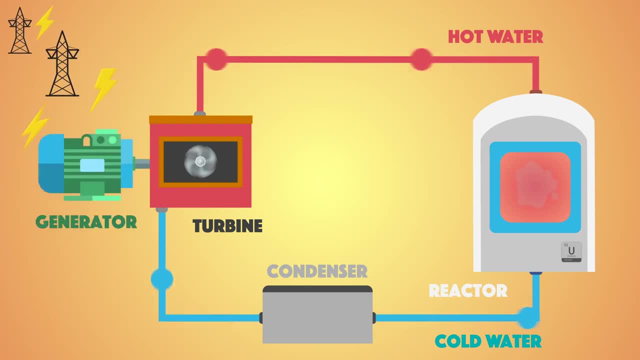 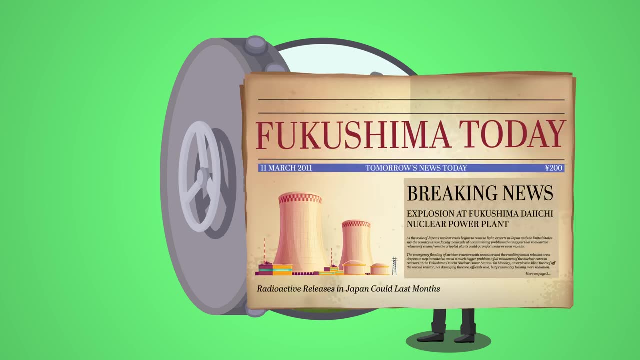 You guessed it: Electricity. Now, this sounds simple, but the complexity begins when making this process safe. We've had two pretty bad accidents in the past: Fukushima and Chernobyl. These both caused thousands of casualties and effectively killed thousands of people. But what's the difference between? 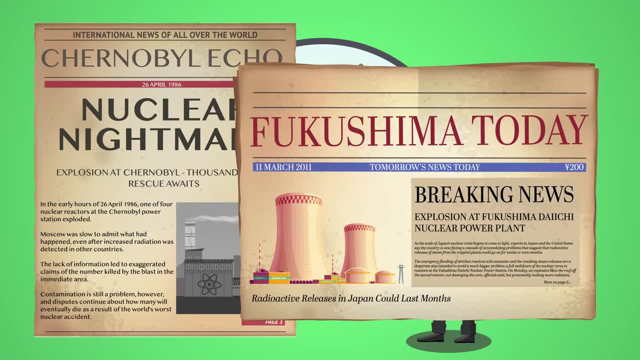 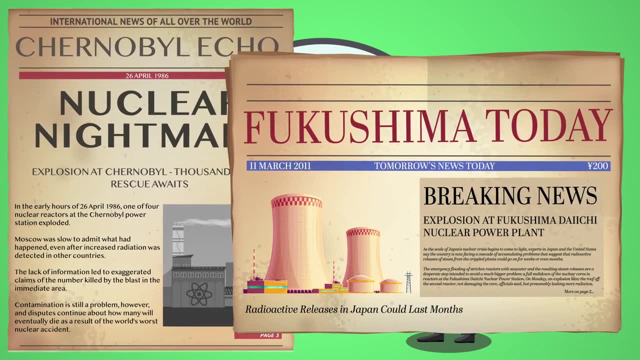 the two. Well, nuclear energy has affected millions of people. There are some good videos on YouTube that explain what went wrong on those days, what nuclear engineers have learnt from it and, ultimately, how we can ensure nothing on this scale happens again. Nuclear energy. 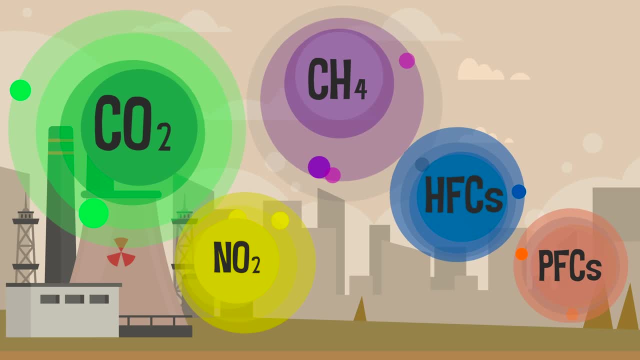 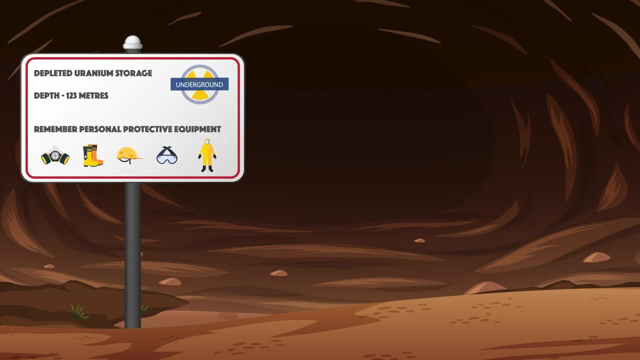 is favoured today because it doesn't release any greenhouse gases, but instead produces radioactive waste. Now, this is deadly stuff and needs to be stored deep underground for some years before it's considered safe. So this takes us back to our earlier question: How can we take mankind into the future? Well, 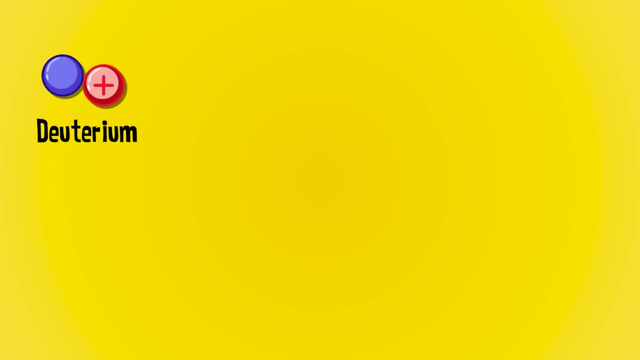 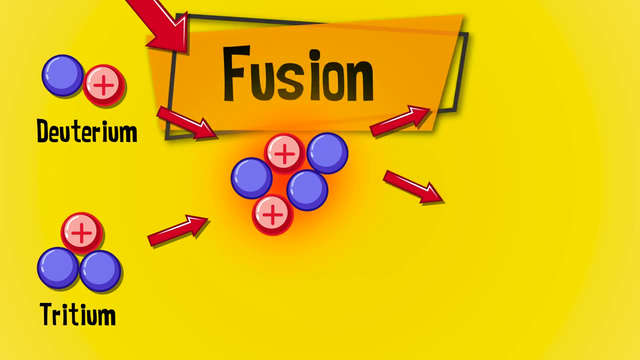 instead of splitting atoms, what if we fuse them together? Well, our sun does exactly this. Remember when we briefly mentioned fusion. Well, this is it: A new type of nuclear power With very little waste and almost free energy for everyone. the possibilities for this is: 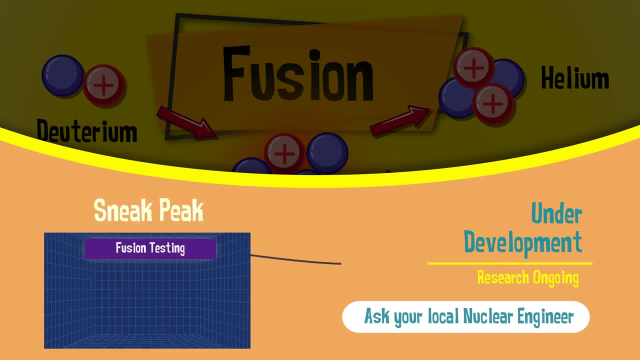 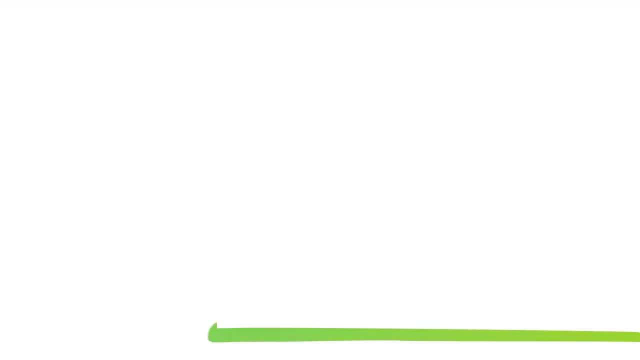 unreal. What we learnt from simulating nuclear explosions can bring us closer to understanding fusion and put this power on the grid, making these possibilities real. Aside from trying to bring free energy to everyone, nuclear power can also be used as a source of energy. 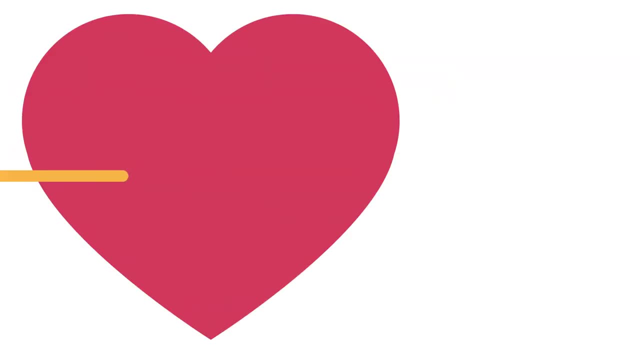 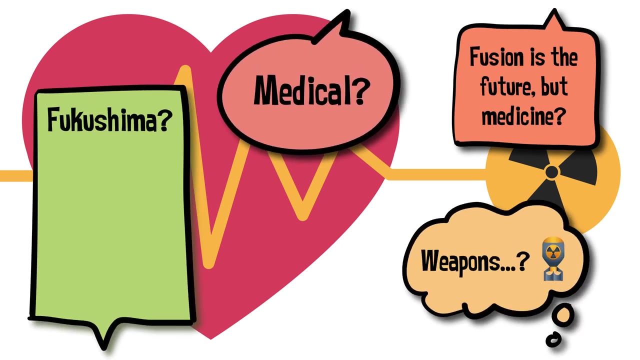 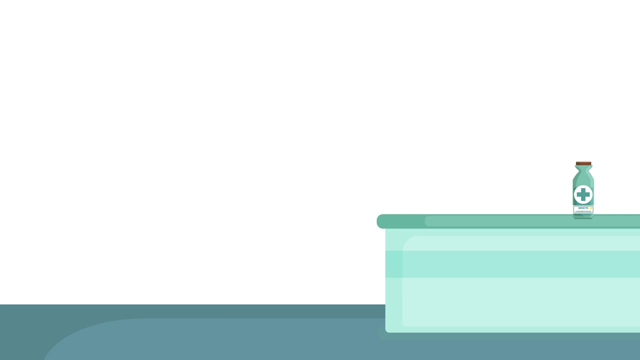 I know what you're thinking: Weapons of mass destruction, Fukushima and Chernobyl. How could they possibly operate in the medical industry? Well, they continue to look into how small, controlled amounts of radioactive material can help patients, like making cancer show up better on scans or even treating it altogether.